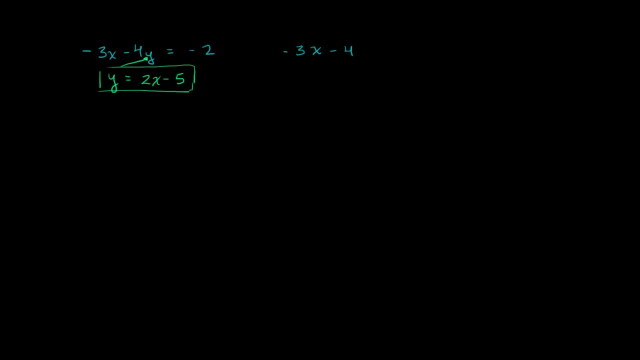 but instead of putting a y there, the second constraint tells us that y needs to be equal to two x minus five. So it's four times two x minus five, two x minus five, and all of that is going to be equal to negative two. 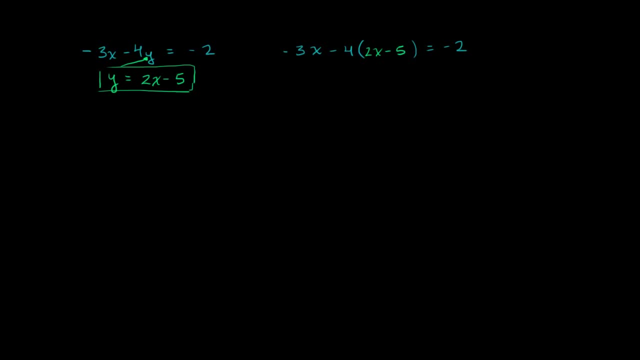 So now we get just one equation with one unknown, and now we just have to solve for x. So let's see if we can, if we can do that. So it is negative three x, and then this part right over here, we have a negative four. 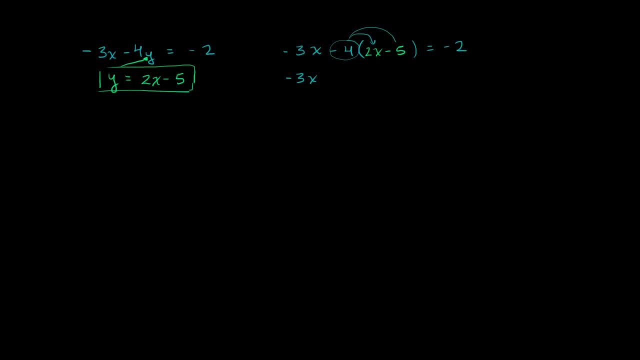 We'll be careful. right over here We have a negative four that we want to distribute. We're gonna multiply negative four times two, x, which is negative eight, x, and then negative four times negative five is positive 20, and that's going to equal negative two. 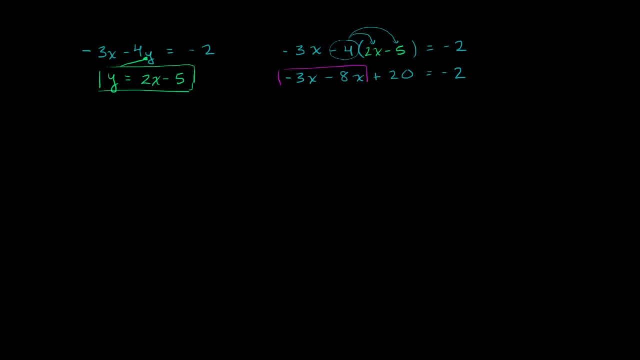 And now we can combine all of the x terms, So negative three x minus eight x, which is going to be negative 11 x, Negative 11 x, and then we have plus 20.. Plus 20 is equal to negative two. 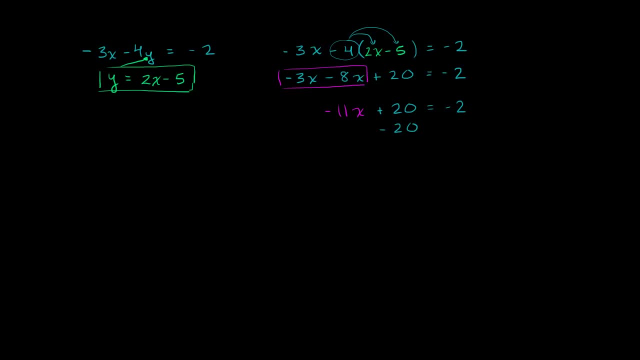 Now to solve for x. we'll subtract 20 from both sides to get rid of the 20 on the left hand side. Subtract 20 from both sides. On the left hand side, we're just left with the negative 11 x. 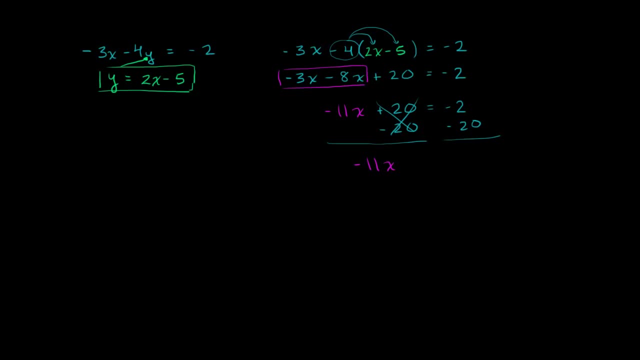 Negative 11, x. And then, on the right hand side, we are left with negative 22.. Negative 22. Now we can divide both sides by negative 11.. Negative 11. And we are left with: x is equal to 22. divided by 11 is two. 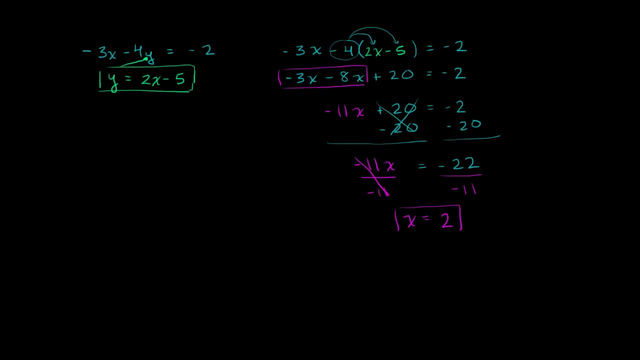 and the negatives cancel out, x is equal to two, And so we're not quite done, yet We've done, I guess you could say, the hard part. We've solved for x, but now we have to solve for y. 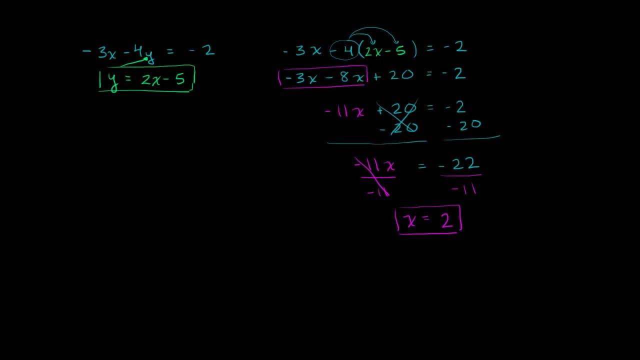 And we can take this x value into either one of these equations for y, But this second one has already explicitly solved for y, So let's use that one. So it says y is equal to 2 times instead of x. we now know that the x value where these two intersect. 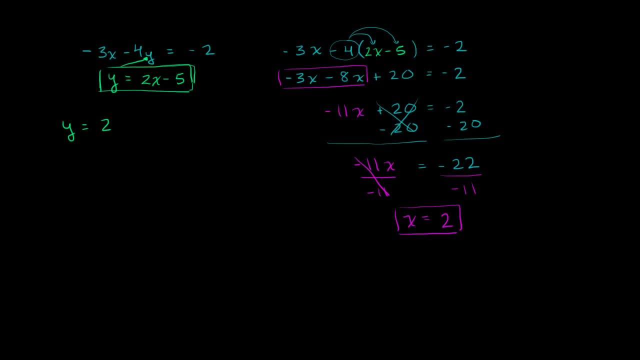 you could view it that way- is going to be equal to 2.. So 2 times 2 minus 5.. Let's figure out the corresponding y value Minus 5.. And so you get: y is equal to home stretch. 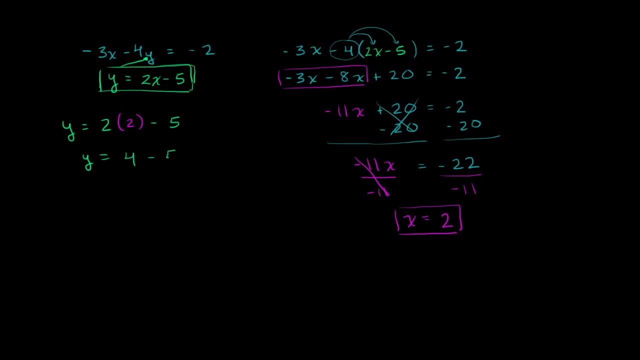 y is equal to 2 times 2 is 4 minus 5.. So y is equal to negative 1.. And you can verify that it'll work in this top equation If y is equal to negative 1 and x is equal to 2,. 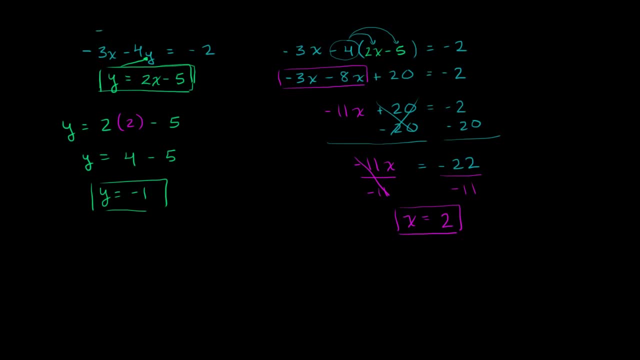 this top equation becomes negative 3 times 2,, which is negative 6, minus 4 times negative 1,, which would be plus 4.. And negative 6 plus 4 is indeed equal to negative 5.. So it satisfies both of these equations. 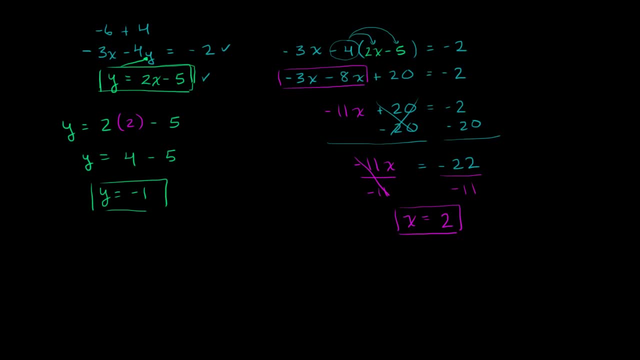 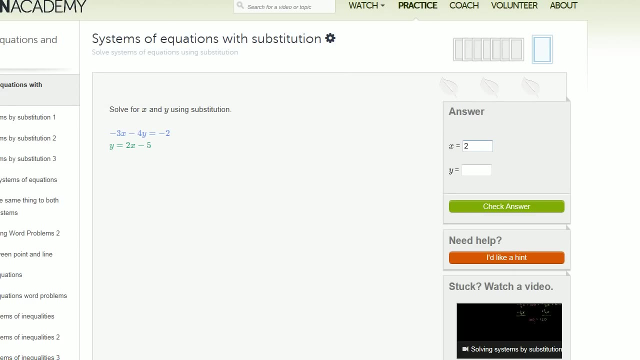 And now we can type it in to verify that we got it right, although we know that we did So. x is equal to 2,, y is equal to negative 1.. So let's type it in: x is equal to 2, and y is equal to negative 1.. 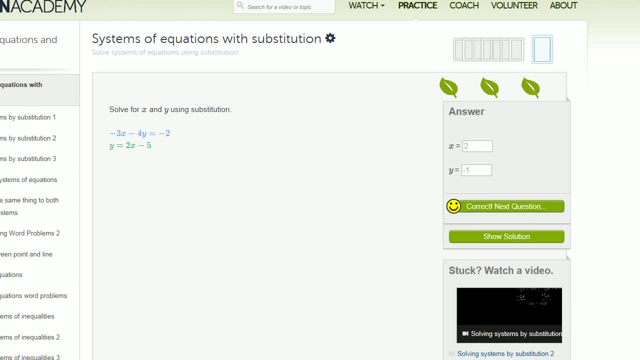 Excellent. Now we're much less likely to be embarrassed by talking birds. 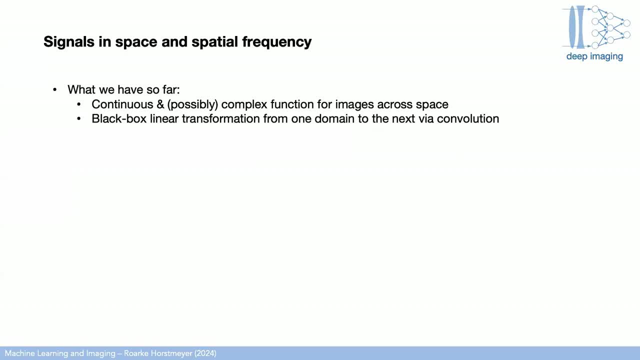 If you've taken signal processing, we've talked about continuous and generally complex functions And we've talked about black box transformations, So hopefully some of these terms are ringing a bell. You haven't taken signal processing for a while. The analogy again is these time, varying signals. 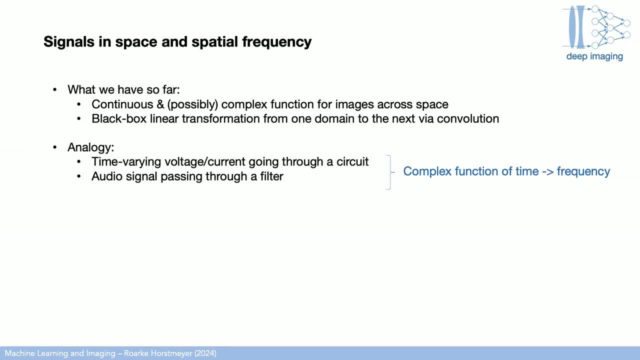 either voltage or current or audio, which hopefully some of you have learned about before. If you hear any of these terms or see them, the first thing- or hopefully what's coming to mind- is the idea of a Fourier transform right, And so Fourier transforms of functions across space right.